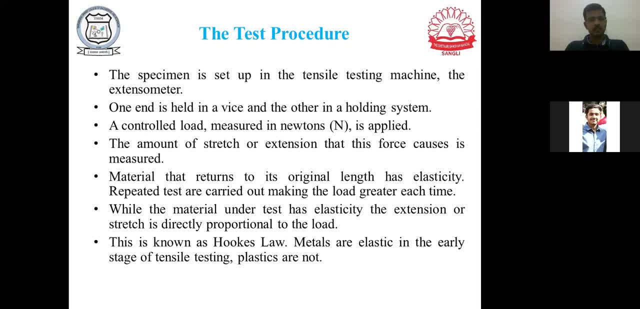 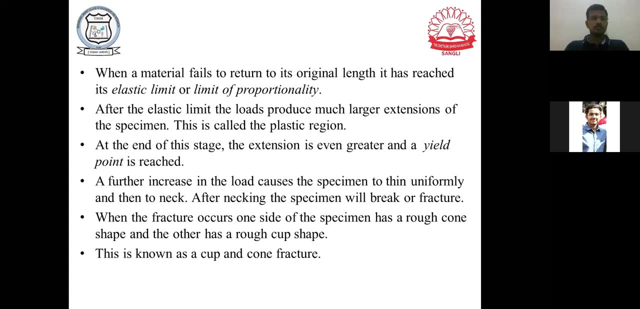 So obviously after a certain time that material or that specimen is going to fail. And how it is going to fail, that we have discussed yesterday first thing. The second thing, very important, is that during that fracture or during that failure, whatever resistance that material shows to failure is nothing but the tensile strength. 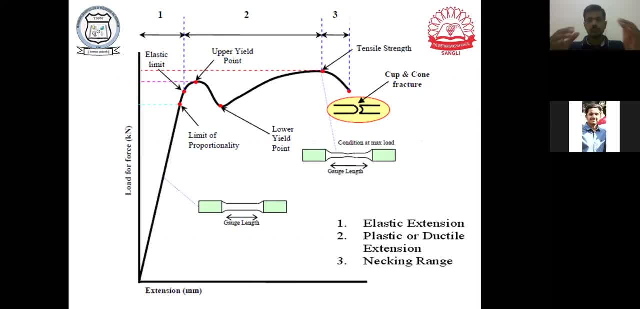 So on the basis of that test, this particular graph can be drawn. Now, how this is done, that we will discuss. That means we will conduct or we will just discuss, just like practical for this tensile testing. I am saying directly practical, So consider this as a practical session. 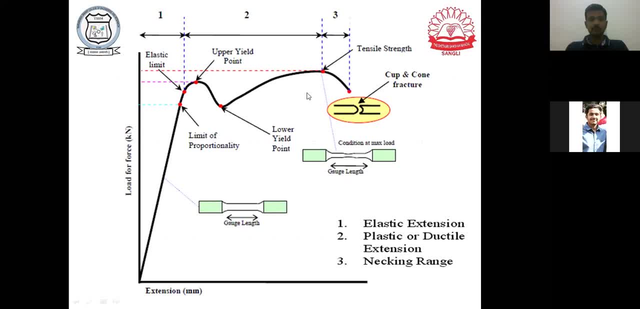 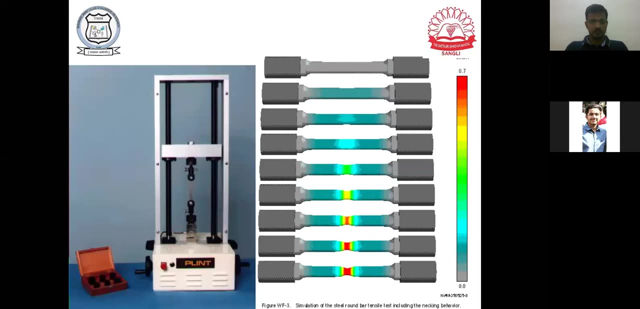 So we will conduct in 20 to 25 minutes, or we will discuss in 20 to 25 minutes how this tensile testing is actually carried out And how it actually works, How that actually making take place, How that material fails. that we will try to discuss. 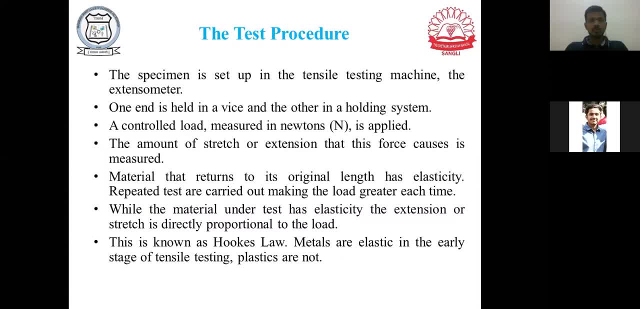 First thing, I will repeat the procedure of the tensile testing and then we will go for that practical of tensile test. So this tank, whatever the specimen, it may be a rectangular shaped or it may be of circular shape- It is fixed in the machine. 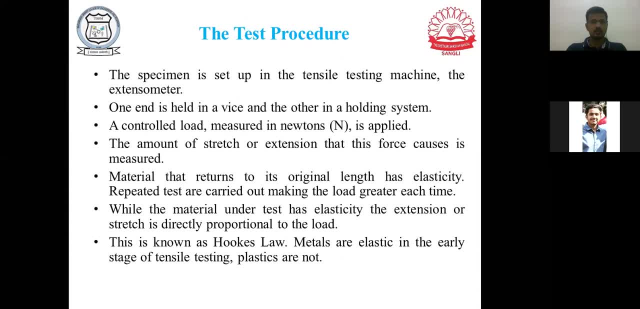 So one end of that specimen will be held in a vice and one will be held in the holding system provided by that machine. And then, after holding properly that particular specimen in the machine, what you need to do is you need to just apply a control load on that specimen. 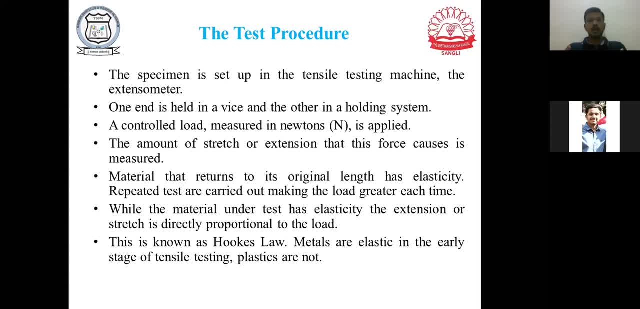 okay, so obviously that load will be in newtons. okay, so after applying the loads, naturally the material or the specimen will lead to extension. that means that particular material, that specimen will stretch. okay, due to the force application. okay, now, in this case, if you apply a small load, 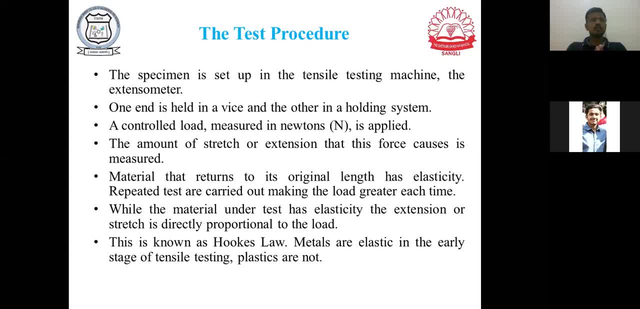 and if you release that load, that material will come back to its original length or material will come back to its original shape. now, this happens due to elasticity, because every material have more or less elasticities, elasticity- okay. so that elasticity, or within that elastic limit, that material regain its original shape after releasing the load on it? okay, now this is: 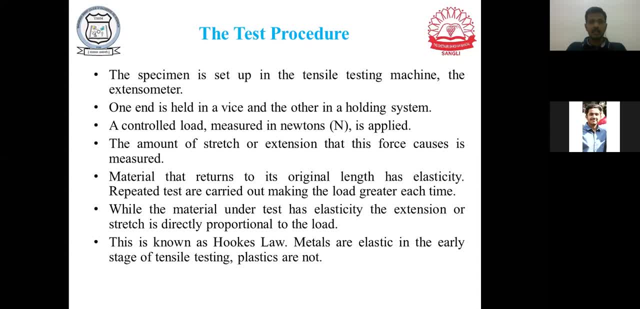 because in this particular case, within this limit, we are getting stresses directly proportional to strength. okay, this is first case, but this is not tensile test. okay, so in this particular case we are getting stresses directly proportional to strength. okay, we have to go beyond elastic limit, we have to enter into plastic deformation, we have to go. 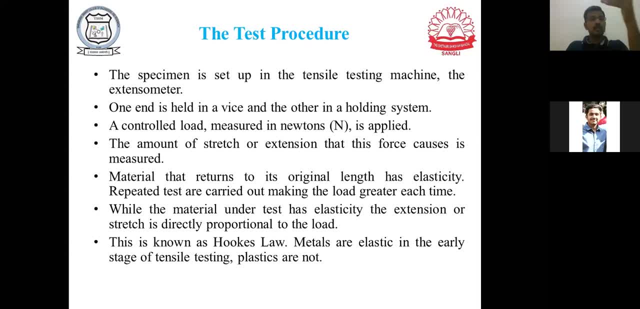 beyond your yield point. you have to go beyond the tensile strength then, and then only material will fail if. if that material is not failing, that means you are not going beyond the tensile strength. okay, so you have to cross the ultimate tensile strength of the material so that the material will fail. 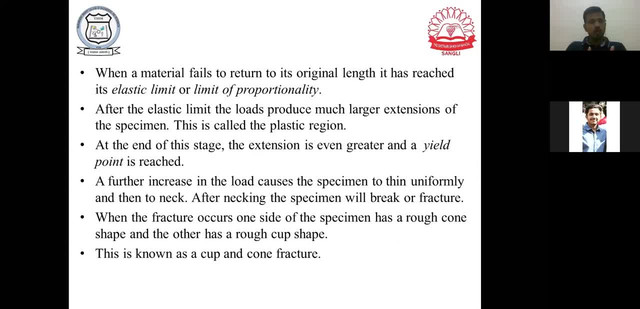 finally, okay. so what you need to do is you go on increasing the load, as you go on increasing the load, as you go on increasing the load. obviously, initially the material will be in elastic limit. after a certain time it will reach its yield point and we know that, after yield point, what will be? 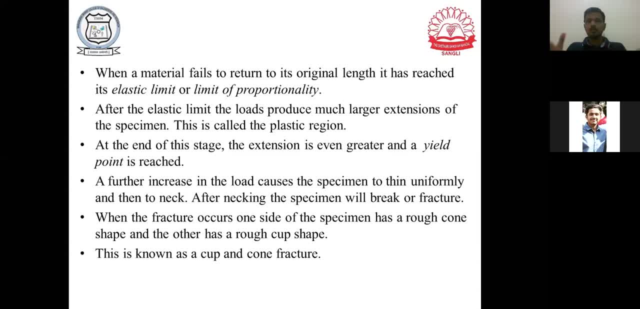 there material will leave its elastic limit and it will enter into plastic region, or it will enter into plastic deformation region. once it enters into plastic deformation, now if you, even if you release the load on that material, that specimen, it will not regain its original shape. that means after: 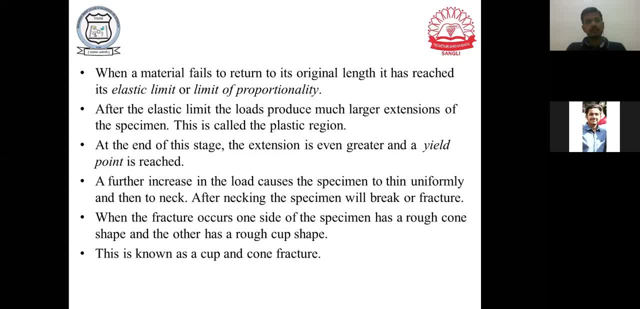 elastic limit. whatever changes that has been taking place into that material, into that specimen, those changes will be permanent. now, now the shape of that specimen is changed because we have entered into plastic deformation region. the specimen's shape is changed, specimens dimensions are changed. this change is permanent now, okay, still, you need not to stop there. you go on increasing the load. 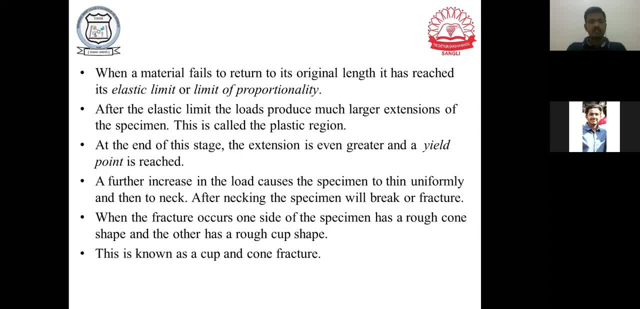 after a certain time, what will happen? that material will stretch straight stage and after a certain time, uh, one point will come there which will result into stretching. that means stretching of that particular material will end okay and making of the, that component, that specimen, will start okay after making certain, after certain time, material will lose, or material rather, instead of losing. i 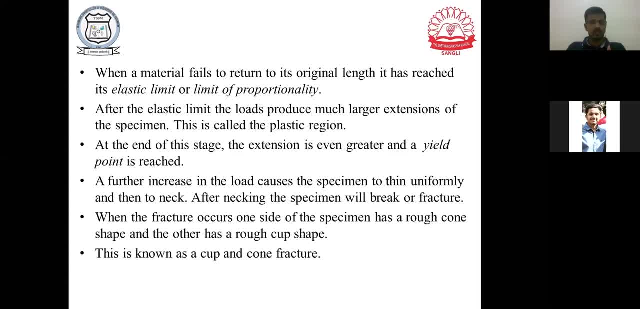 i will use material will end its resistance- okay, resistance to that inside load and it will result into failure. or in other words, you can say it will result into fracture. okay, the fracture which is usually occurred in case of your tensile test is usually cup and cone fracture, but 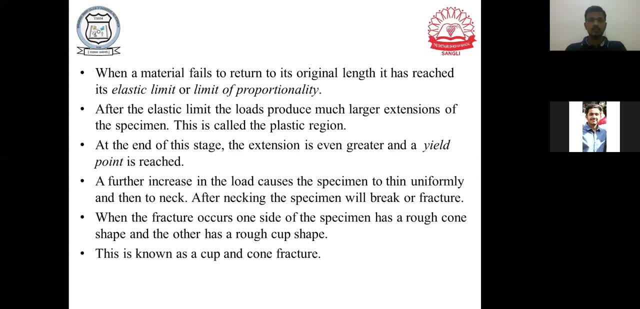 if you are using a ductile material, then, and then only, you will find this cup and cone fracture. this last sentence in this slide you can see over here: cup and cone fracture. okay, so this cup and cone fracture is usually observed in materials which will show some ductility. 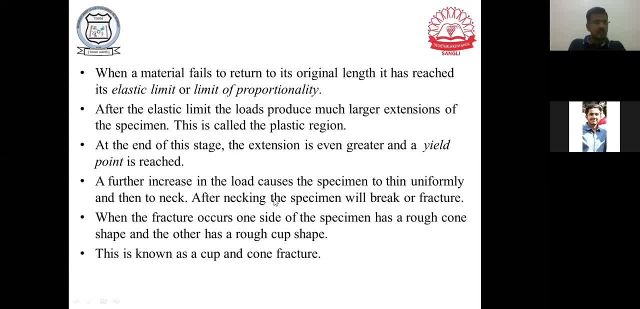 if there is suppose, if there is no ductility, definitely there will be brittleness. and if there is a brittleness, material will not fail in ductile manner, it will fail in a brittle manner. so that will be brittle fracture. okay, we are not going to check brittle fracture, we are 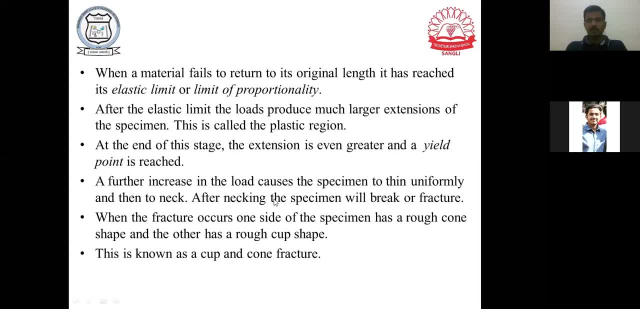 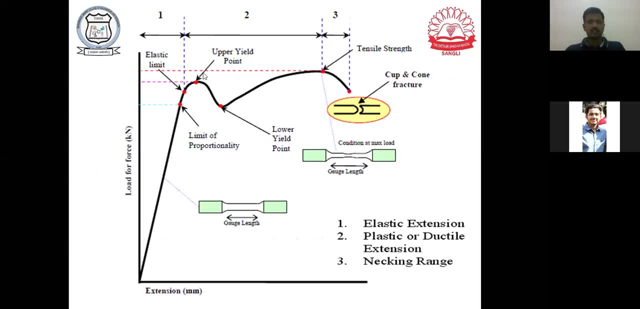 going to check ductile fracture. how, uh, a ductile material fails, how it, how it forms cup and cone fracture. that will this so okay, so this is the graph that we discussed yesterday. again, i am discussing in view of practical now. okay, so this different ductility will not fail and it will not. 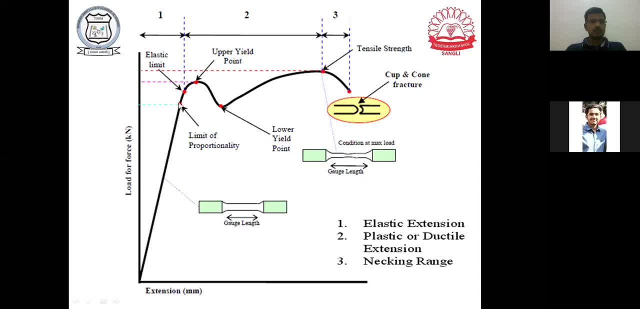 first straight line is nothing but the elastic limit or elastic region. you can see, within this time, even if you release the load, okay, okay, one minute, okay. so during this particular region, okay, even if you release the load, okay, it will regain its original shape because this is a elastic, this is within elastic limit. after crossing this, 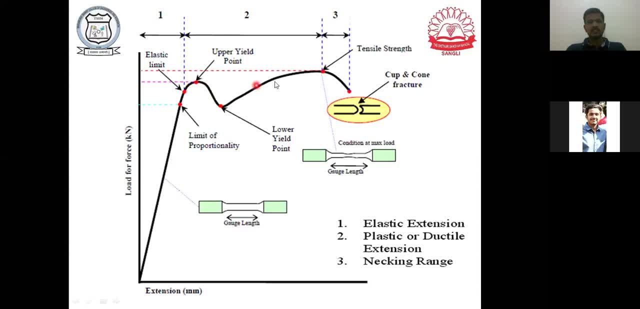 there will be yield point and after crossing yield point there will be plastic region or you can say plastic deformation. this deformation or this region will change the shape of the specimen and that change will be permanent after certain time. there will be a tensile strength- okay, and 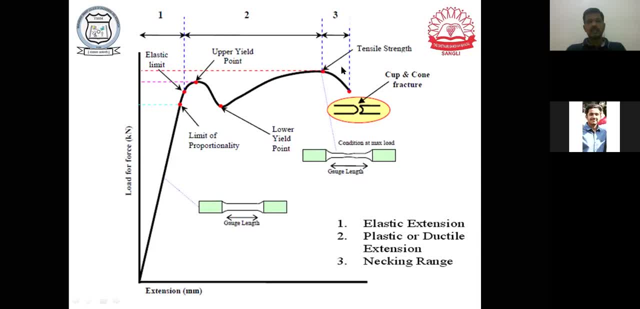 then, finally, after crossing that tensile strength- okay, ultimate tensile strength- finally material will fill. so this end point shows the failure over here you can see in this yellow block: okay, this is the failure. and this forms, if the, if the material is ductile, this forms a cup and cone type of structure, something 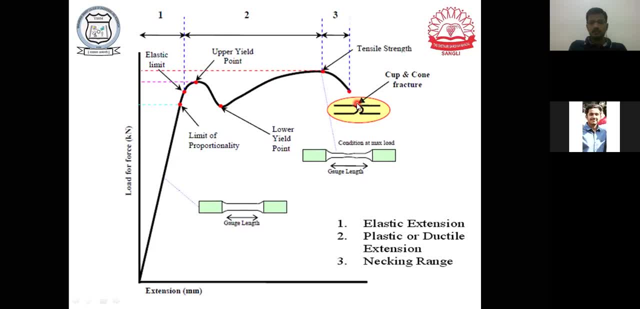 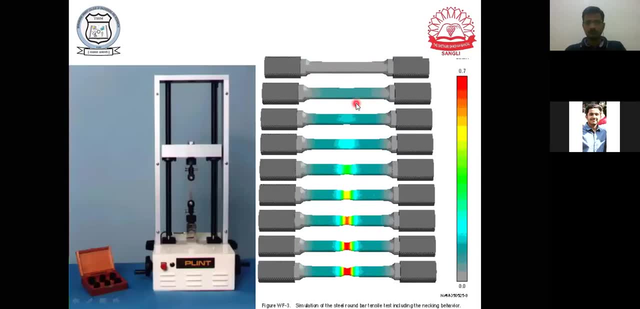 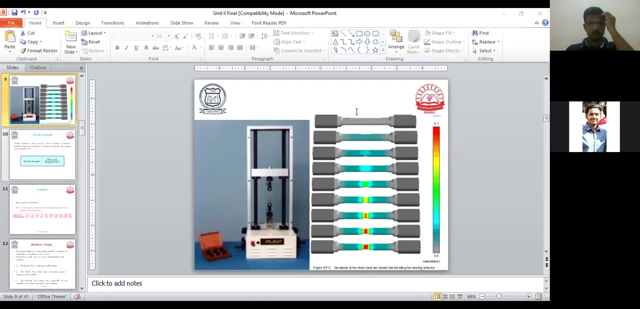 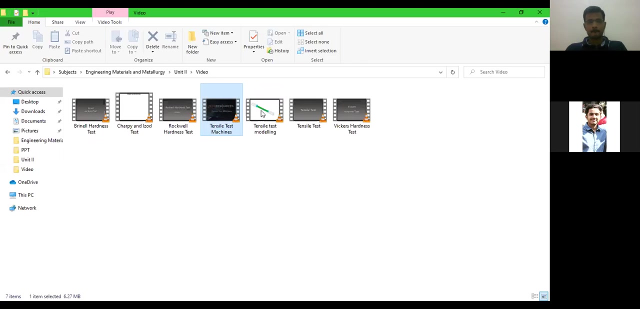 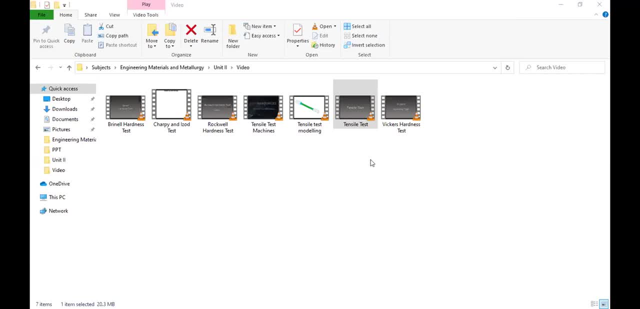 Is it visible? No, sir, video is not still visible. Okay, wait a minute. Folders are visible, sir. Folders are visible. Folder is visible, Am I right? Yes, sir, Okay, wait a minute. Wait a minute. I will directly share the screen so that you will understand. 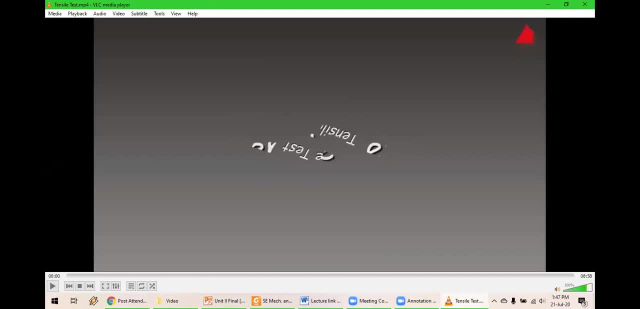 It is started now. right, Yes, sir, it is visible now. Okay, now, look carefully. I will speak in between. Okay, this video. I will try to elaborate the things. Okay, it is self-explanatory video, but still, I will elaborate in video. 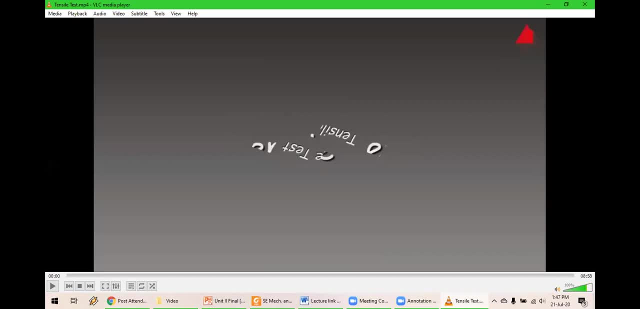 Okay, so try to concentrate on this. This is a tensile test video. Okay, this is as good as performing a practical. Okay, actually, see, the machine that we have is not advanced as shown in this video, But what you need to understand is the basic concept. 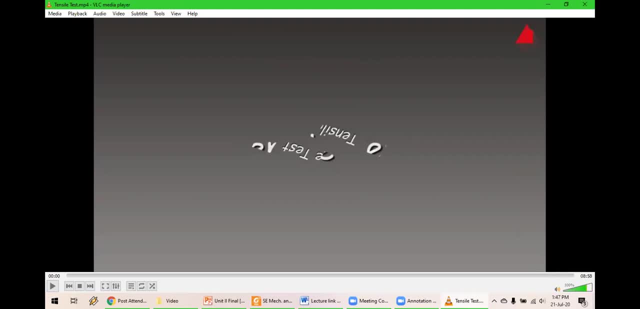 Okay, because, see, in case of the machine that we have, Okay, we apply load manually. Okay, in this particular machine it is directly computer controlled machine and the load is applied through the programming mode. Okay, so I will explain that. Okay, but you need to understand this is advanced machine. 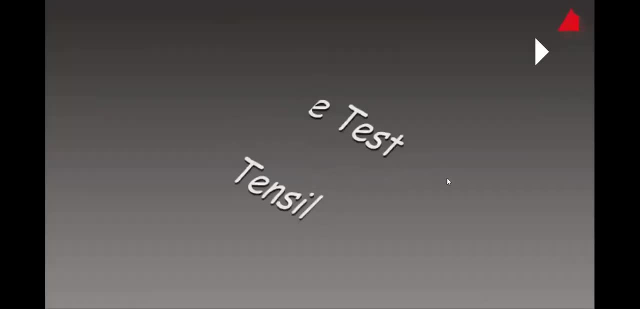 Okay, basically The tensile test. First test: material with yield point phenomenon. Okay, so two tests are conducted in this video. Okay, the first test is conducted for a material, For a material which shows yield point phenomenon, Where it shows upper yield point and lower yield point. 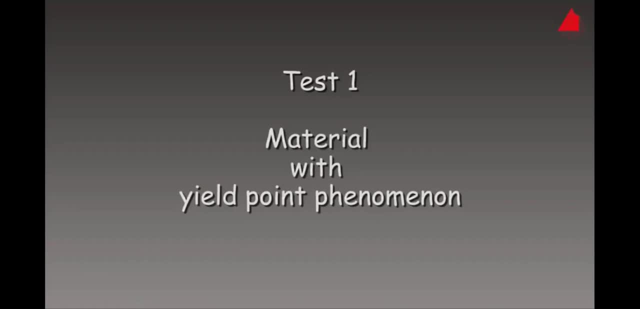 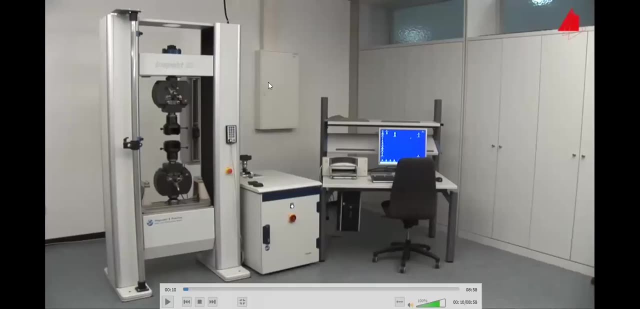 That kind of graph. Okay, it is explained in this video also. We will elaborate that also. Okay, so this is machine. Okay, wait a minute. Okay, this one is the machine. Okay, this one, Okay, and this machine is attached to this computer. 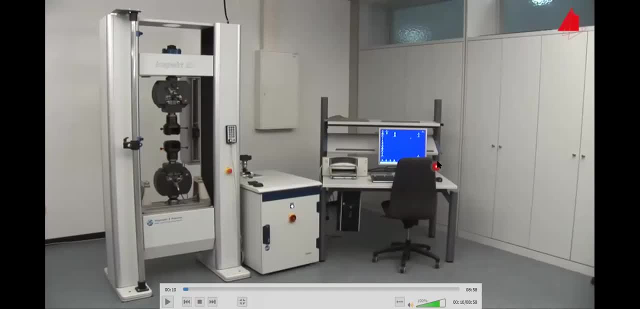 So obviously, the machine will be controlled by this computer. Okay, Whatever load that you are going to apply, Whatever graphs that you are going to observe, Okay, that will be observed in this computer. Okay, I mean on the computer screen. Okay, and the specimen that you are going to say fit. 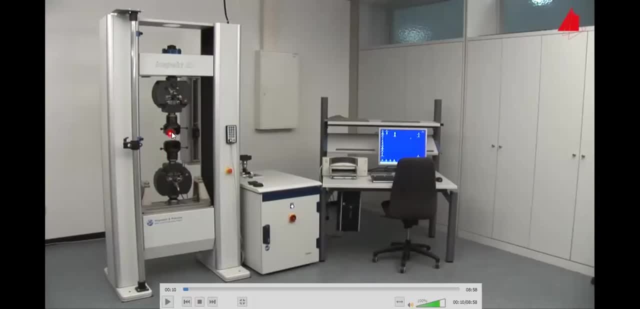 Okay, or that you are going to hold in. the machine will be in this, These two wise Okay. one is holding system and one is wise Okay, so I will play this. So try to concentrate how the specimen is Okay. so let me try this. 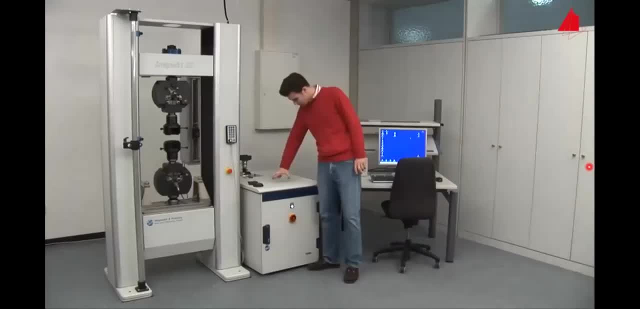 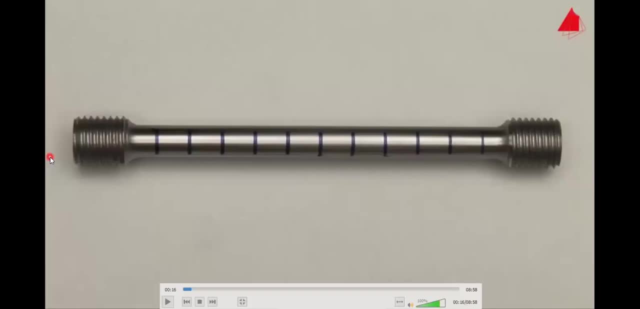 Here we go. So you have a cylinder builder here. Okay, where is this cylinder coming out of the inside of the cylinder? Okay, I will put this cylinder back to固定 and then I try to put the cylinder back to固定. 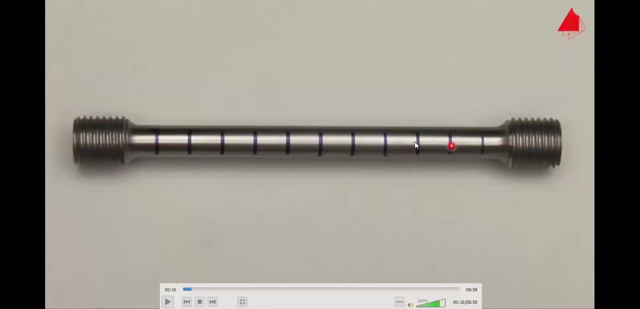 Here in the cylinder At the end of, there is a cylinder unit with Q1 when it is in the bath And then the cylinder is at 50.. can see over it now. this is to just to understand, uh, where exactly the necking is going to start, or? 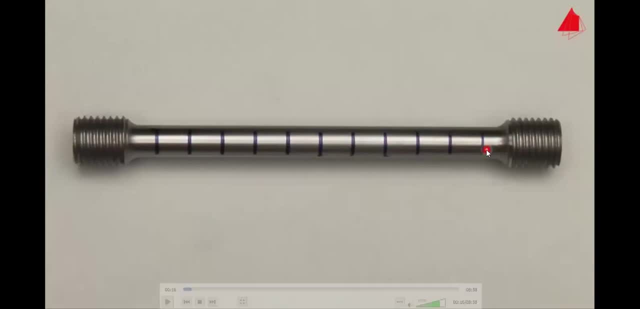 how it is extended, that that will be, uh, probably uh, to analyze that. okay, it will be easy if you mark such lines on the specimen because see whether the stretching is more in this region or more in this region, or this region or this that you can observe immediately after the test. 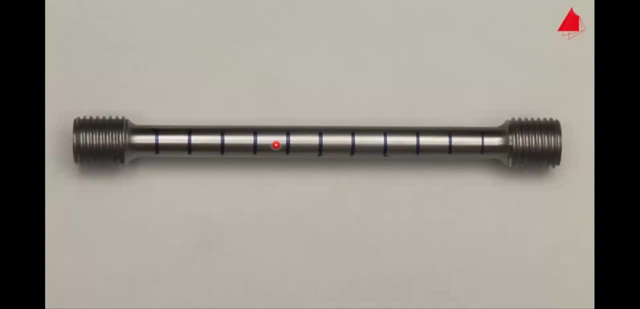 okay. so how it is done, that we'll see now. piece: it has a cylindrical test region with an original diameter of 10 millimeters and an original gauge length of 100 millimeters. okay, so this gauge length is 100 mm. okay, and this diameter is 10 mm. remember this meters within this test region. 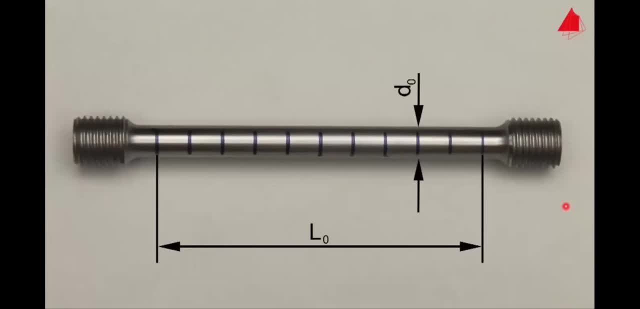 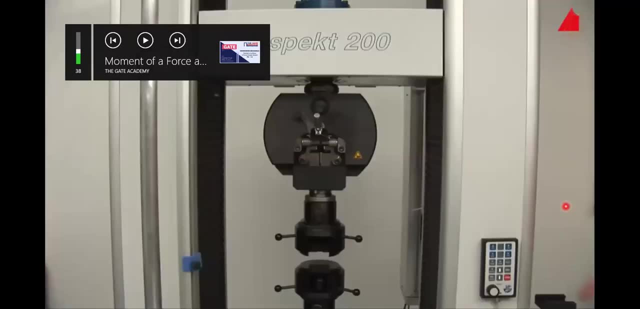 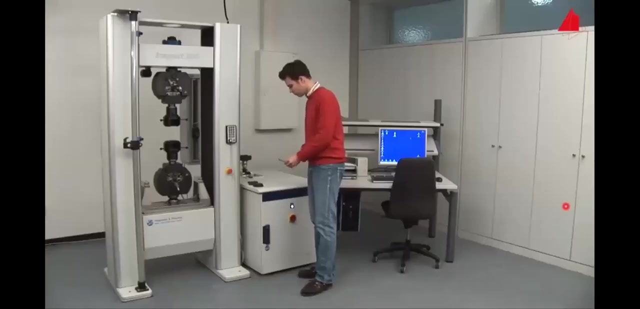 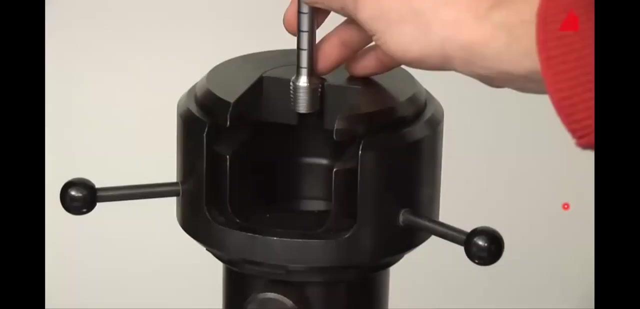 distance marks have been drawn at regular intervals. they help to visualize and measure the plastic behavior of the specimen. using a hand control, the tester moves the upper cross head into its correct starting position. okay, so much now he can set. now. okay, to fit the specimen is the threaded ends of the test piece in the lower and upper grips of the testing. 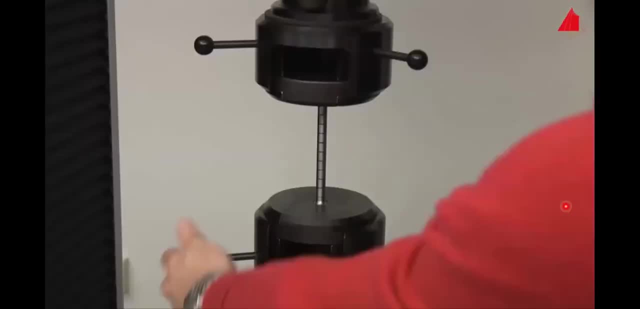 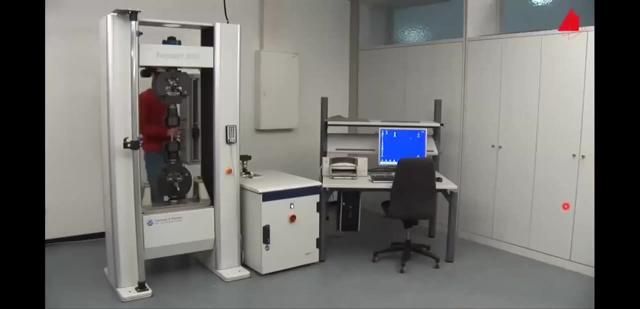 will continue the measurement process. it is okay, so it is fitted. in the next step he swings the extensometer into its working position and checks that everything is correctly prepared. so then he selects all necessary advanced machine to certain sensors and everything is used in this machine. okay, to get the accurate results. okay, retesting parameters on the control computer. 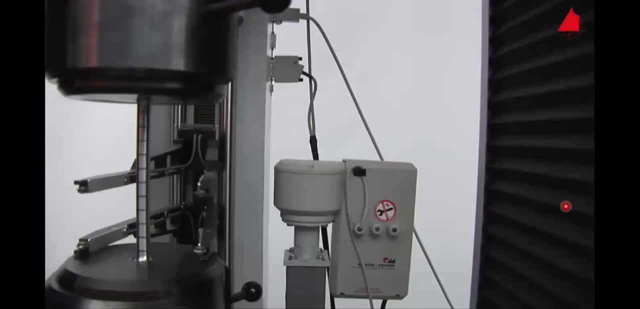 ready, the testing process is done and the experiment is complete. The test starts and the extensometer's sensor arms are carefully pressed onto the test piece. This way the gauge length can be measured throughout the whole tensile test. The gauge length is displayed at the bottom right-hand corner. 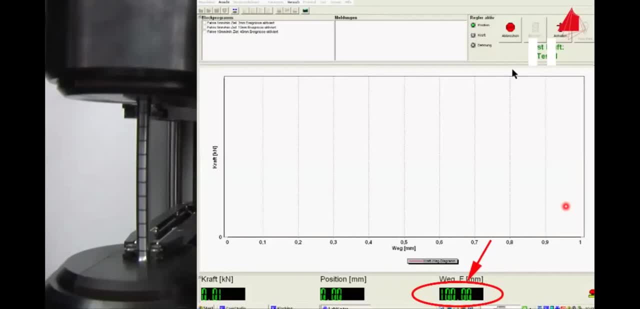 Okay, now this white color on this right side shows the computer screen. That means the load that you are going to apply will affect this specimen And how it is going to affect The graph will be drawn in this particular region. That may be the software of that particular machine. 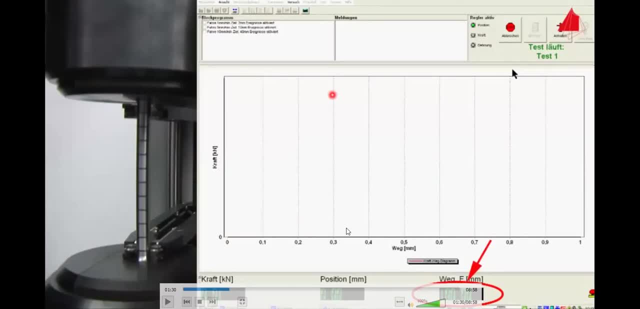 So in that software the graph will be drawn here automatically, So you do not have to do anything, You just increase the load. Now concentrate on this. This is the computer screen and this is the actual machine picture, So it is not like. this is the pause. 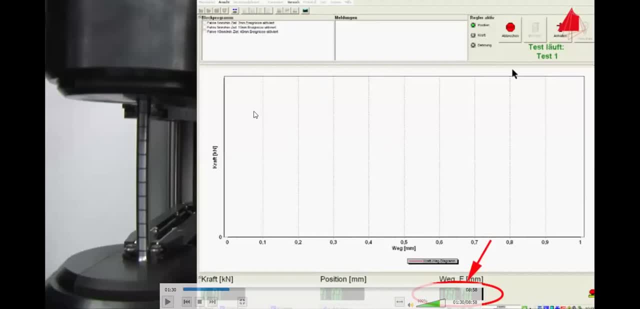 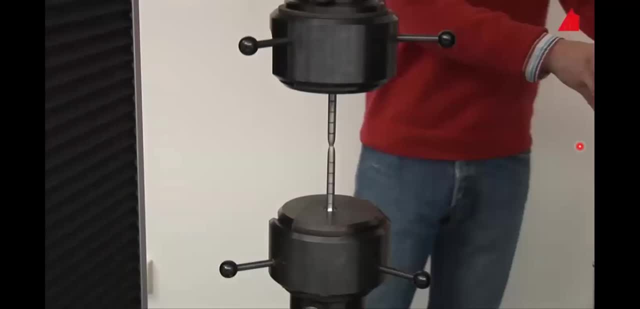 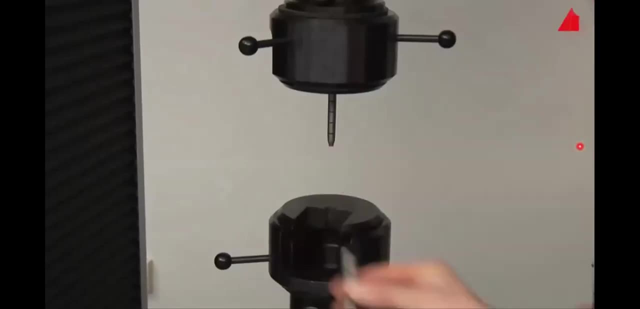 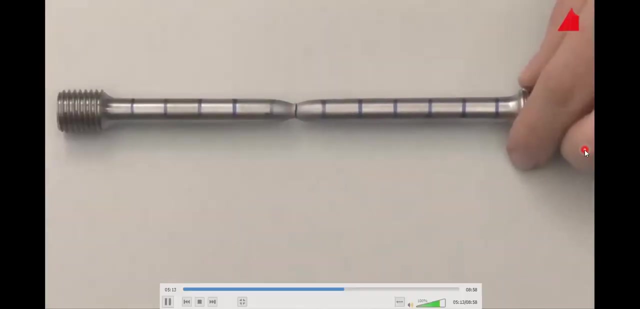 Okay, so it is not like. this is the pause, This is running and the load has been applied here, And whatever the In the last step the tester swings the extensometer back into its resting position and removes the broken test piece On the work table. he puts the fragments back together again. 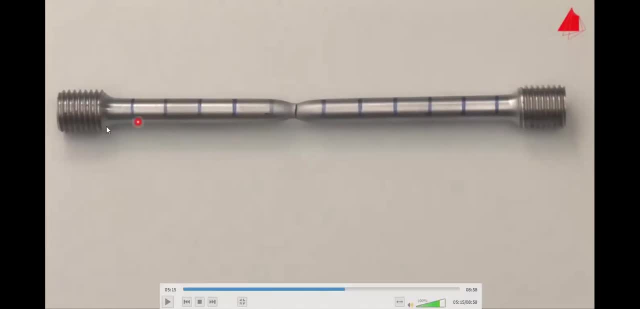 Okay, so this is your broken piece. Now this has been stretched. Okay, because now in the next part of this video, because now in the next part of this video, the original piece will be kept over here. Okay, so you paying. 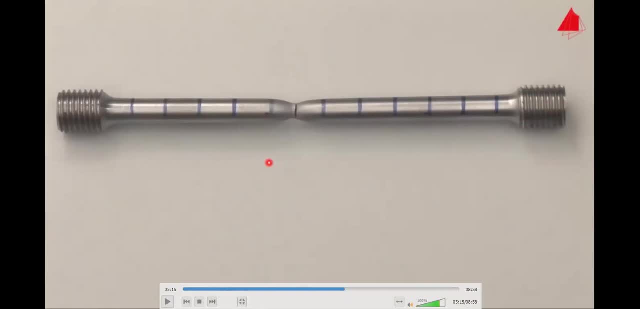 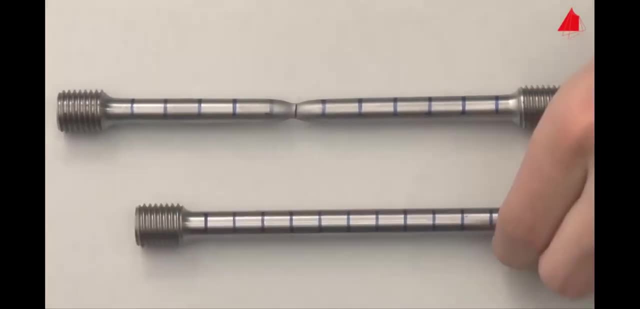 can just compare with the help of the distance marks, the percentage elongation after fracture can be determined. this is the permanent strain after fracture and amounts to about 30 percent. okay, so this was the size of our original uh specimen and this is the fractured specimen. so 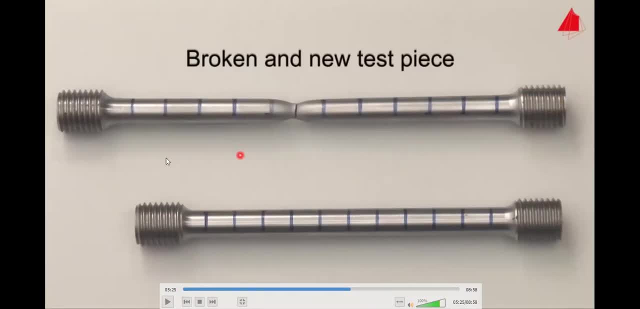 you can see, the elongation has been there, okay, the stretching of that specimen- okay, you can see so, almost almost 10, 20 mm has been increased in this example. please note that the percentage elongation after fracture depends on the length to diameter ratio by measuring the smallest diameter at the 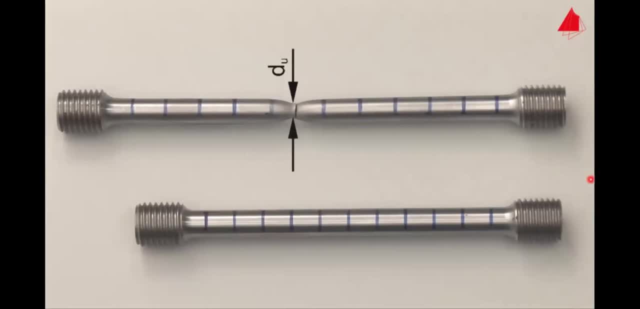 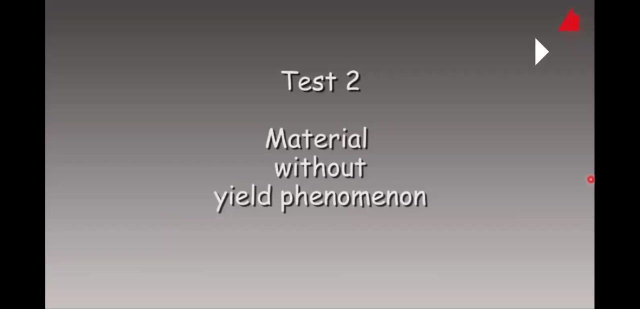 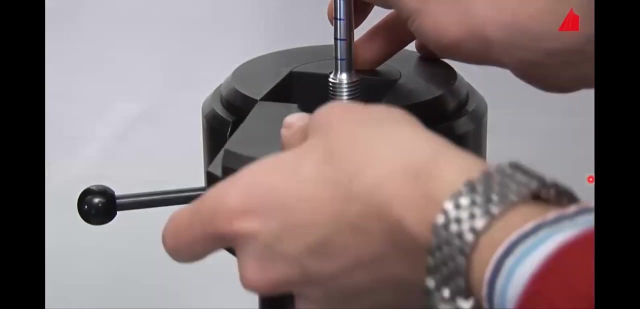 point of fracture, the percentage reduction of area can be calculated. it describes the reduction of cross-sectional area at the point of fracture in relation to the original cross-sectional area in the second tensile test material material is without yield point, without yield phenomenon. okay, in this case it is a precipitation. strengthened aluminium alloy has exactly the same shape and 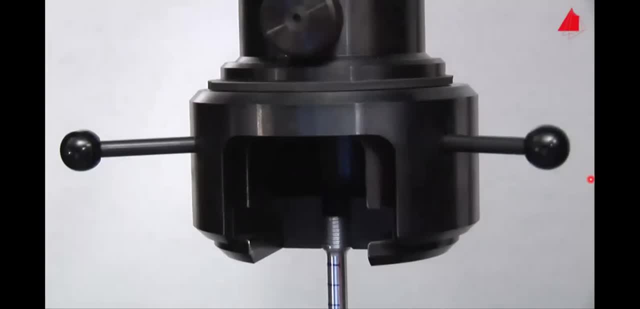 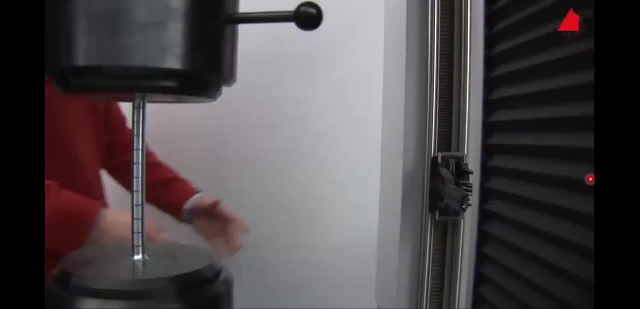 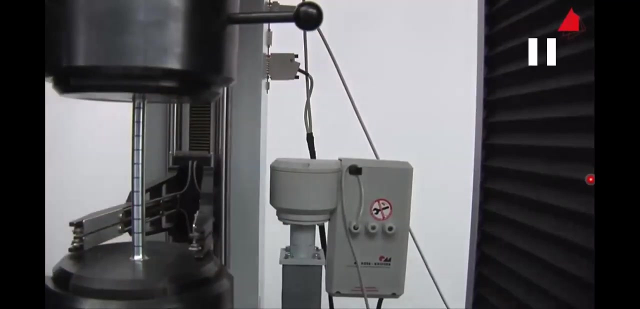 dimensions as the specimen in the first test. it is cylindrical, with an original diameter of 10 millimeters and an original gauge length of 100 millimeters after fitting the test piece. oh, material is different in both the cases. okay, in the first case the material was plain carbon steel. 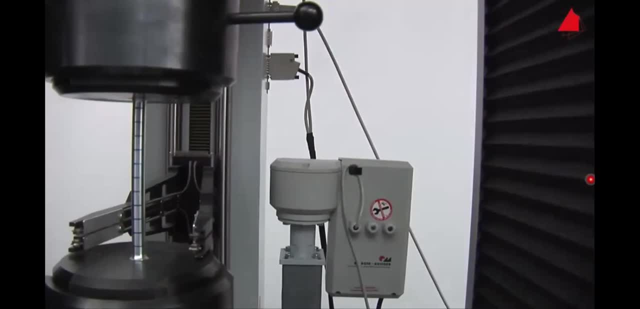 which usually shows higher ductility. okay, and it is a soft material- okay. in case of this aluminium alloy it is- usually shows, uh, lower ductility and more brittleness. okay, not more brittleness in the sense, not higher brittleness, but comparatively it is it. it has more brittleness as compared to the 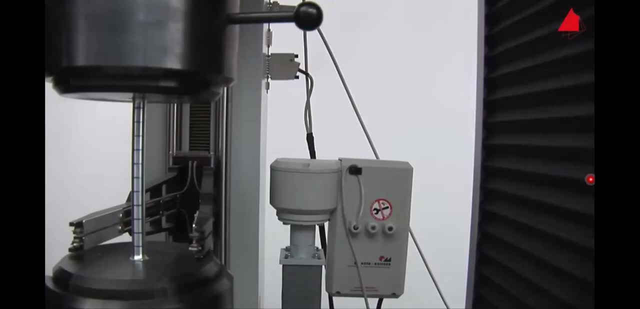 plain carbons: okay, and yield point phenomenon is different in this particular material. it will not reach to uh upper yield point and lower yield point. nothing will happen. okay, it will reach its upper end point and then it will directly start its uh plastic deformation. it will not come back to its uh. 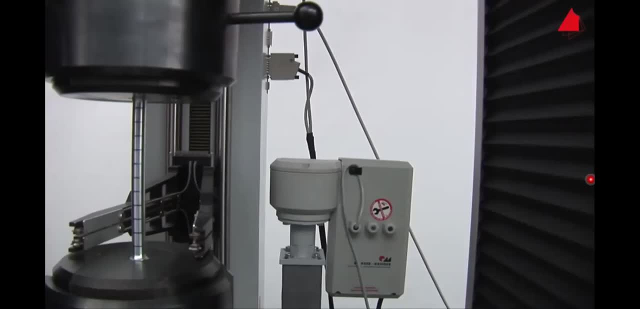 it will not come down to its lower end point. there is nothing like that, no lower end point, and all this. there will be one yield point only, okay, and that will be the yield of that material. okay, you will see that during this particular experiment, the extent summative into its working position. 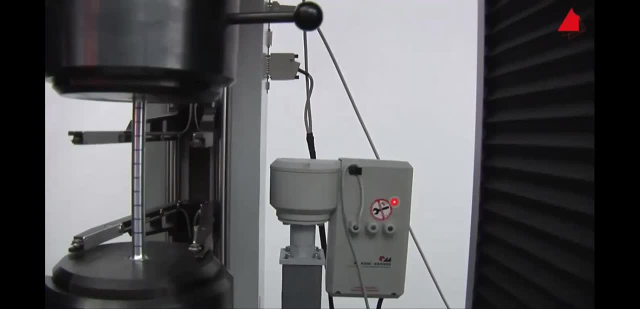 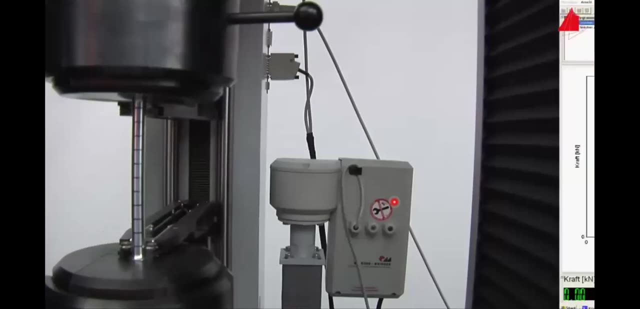 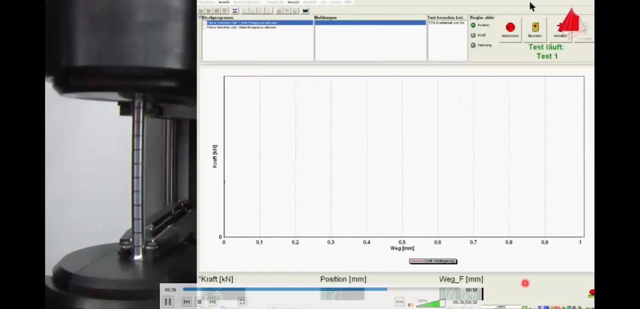 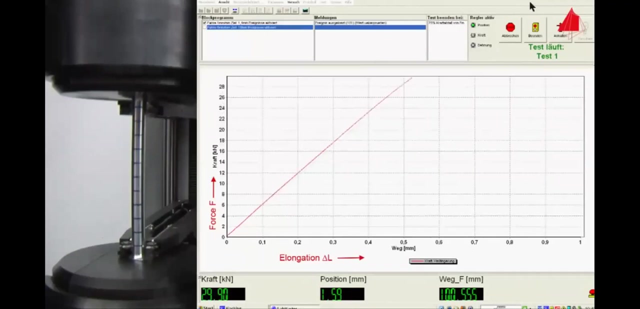 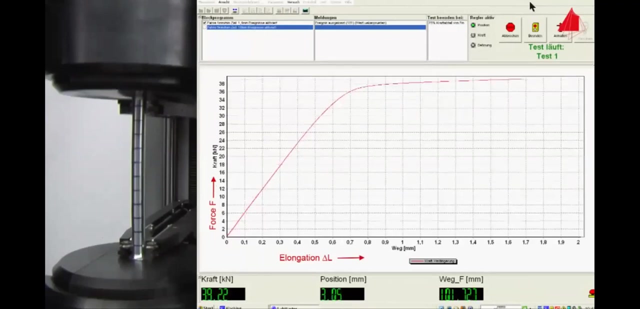 the test can start. the initial linear curve in the force elongation diagram diagram again shows the elastic behaviour of the material, But this time the end of the elastic area is not revealed by a sudden drop of force or any distinct change. So there will not be any kind of sudden jerk of force or sudden drop of force. It will. 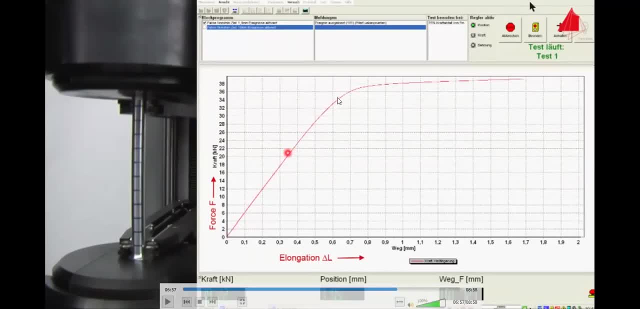 directly. you can see over here. this one is the elasticity up to here or somewhere over here. the yield point will be there And after this yield point it will directly enter into plastic deformation. So there will not be any type of dropping. 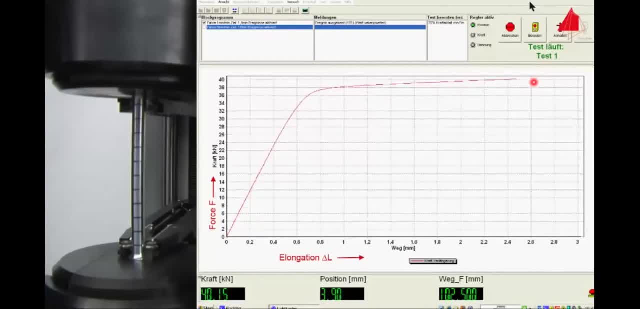 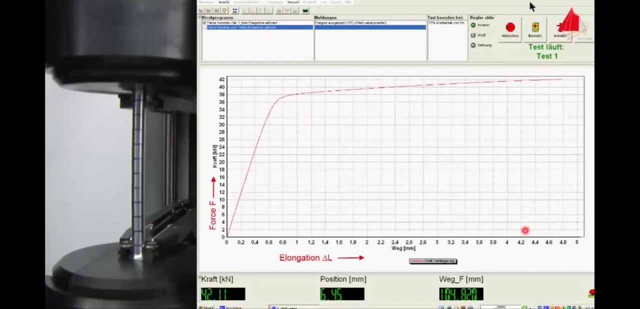 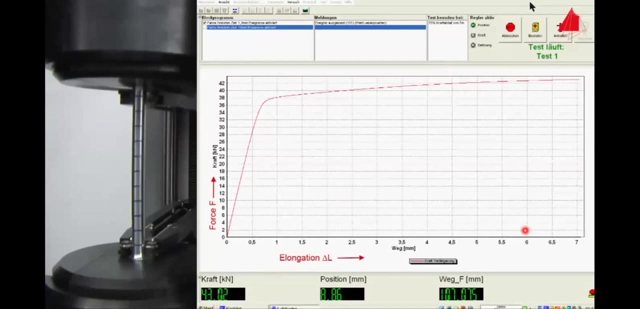 There is a smooth and gradual transition from linear elastic behaviour to plastic deformation. In the further course of the tensile test, the force increases and the test piece again is strained uniformly along its length. At the point of maximum force a neck develops and all subsequent plastic deformation is. 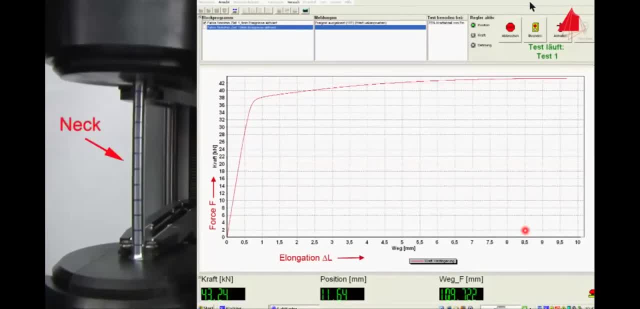 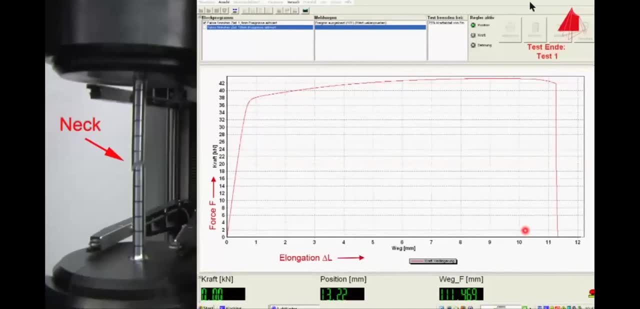 confined to the neck. It will continue straining to this neck until fracture finally occurs there. At this point it will fail. Now you check, there is no necking. There will be necking, but that will be very, very small necking, unlike the last piece You can see over here. 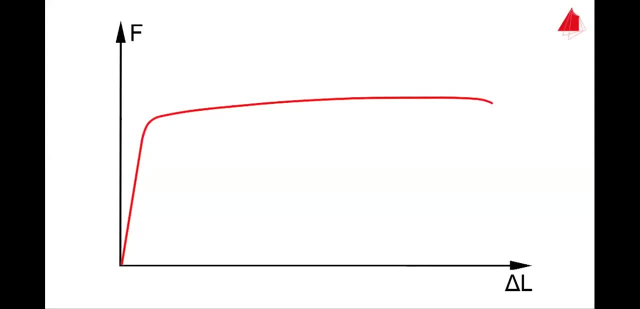 As a common substance, the neck will be very, very small. As a common substitute for the yield strength, the, This will be graphed: for the materials which do not show yield phenomenon, 0.2% proof strength is used. It is the stress that causes 0.2% of plastic deformation in 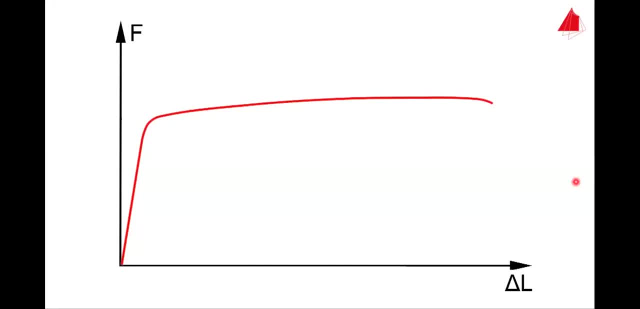 the material. And this is the way to calculate it. First of all, the elongation that corresponds to 0.2% of strain has to be computed For an initial gauge length of 100mm. the length of the neck will be 0.2% of the strain. 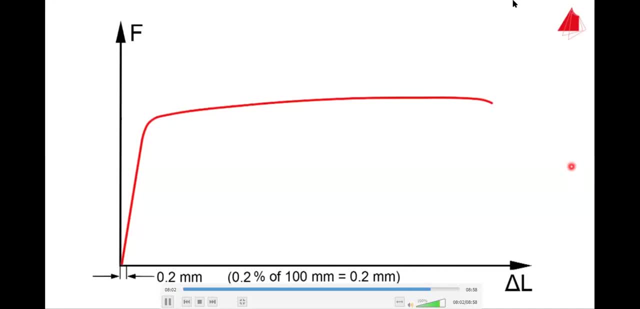 For an initial gauge length of 100mm, the length of the neck will be 0.2% of the strain. For an initial gauge length of 100mm, the length of the neck will be 0.2%. The result is 0.2mm. 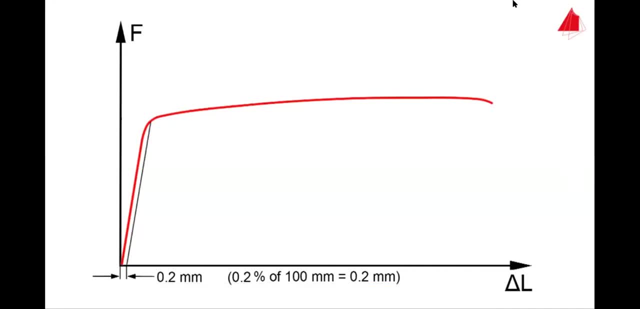 In the force elongation diagram a straight line parallel to the elastic line is drawn through the offset point of 0.2mm of elongation. The force at the intersection point of the offset line with the force elongation diagram is designated as Fp0.2.. 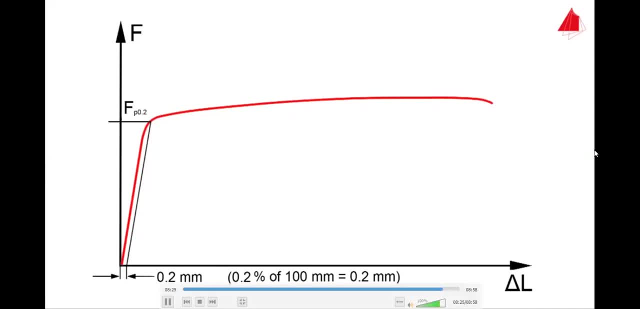 This is the force that causes a plastic strain of 0.2%. The 0.2% proof strength, Rp0.2, is equal to Fpu to FP 0.2 divided by the original cross-sectional area S0. Tensile. 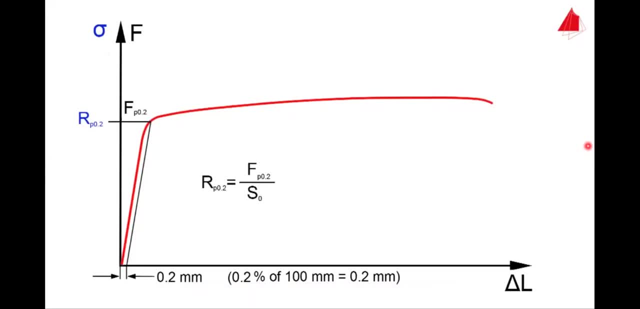 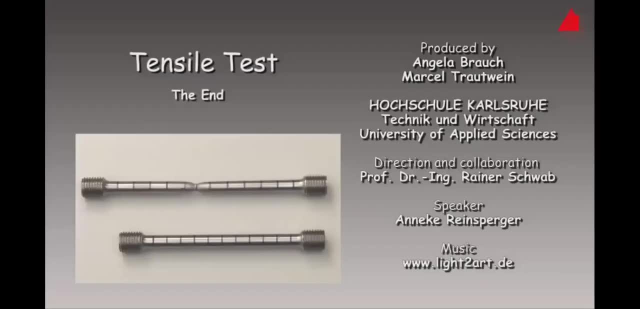 strength, percentage elongation after fracture and percentage reduction of area are calculated in the same way as in the first test. It is very easy. Tensile test does not take much time. You will repeat these things in your form also. So in the solid mechanics now the subject is yours. In that subject also you will.